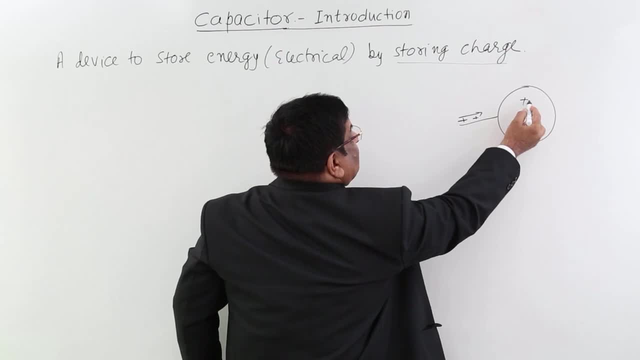 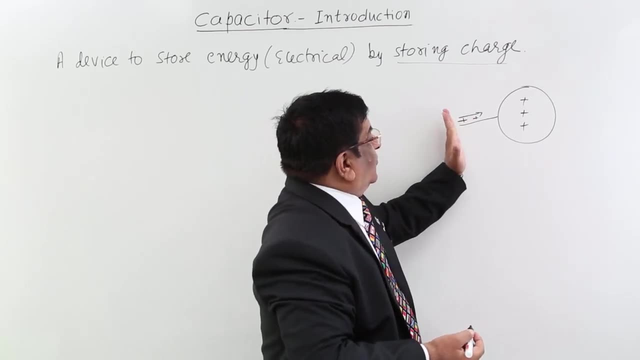 and carry certain charges to it. then the moment I give it certain charges to it, the more charges then these charges will repel it like a spring. Then I have to push it, apply a force, do the displacement and put the charges here. That means I am doing some. 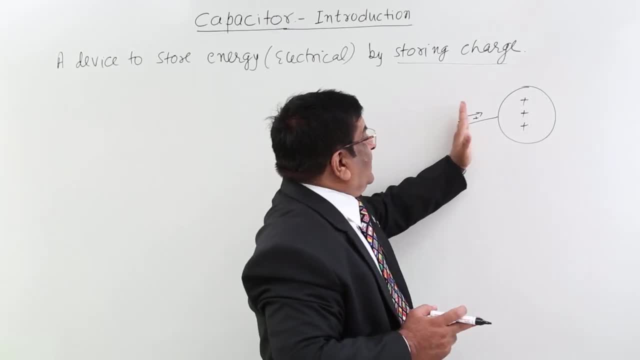 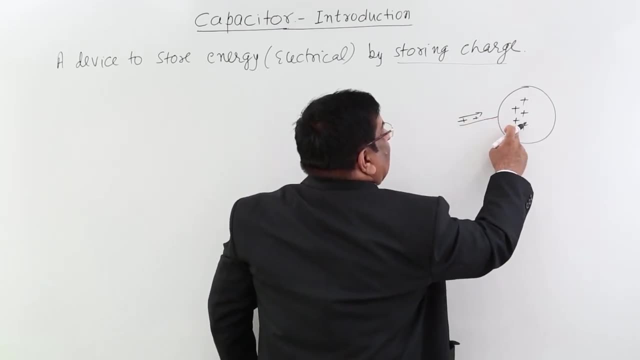 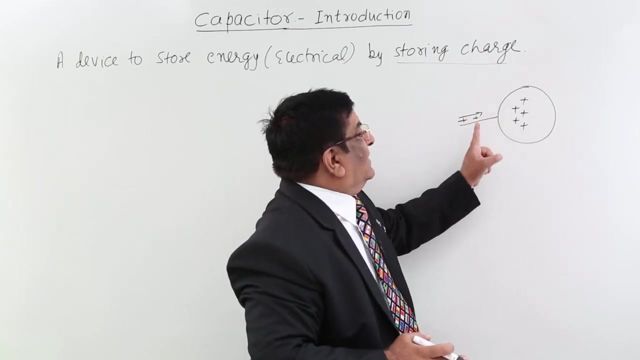 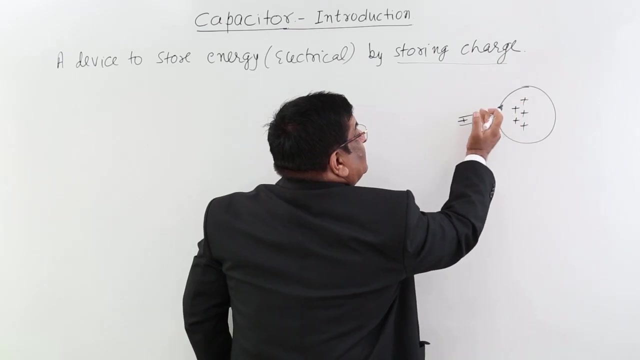 work. I am using my energy in pushing it and after some time I push them here. If I push them here, then my work, my energy, which I have transformed in work to put them here, that energy is stored here. Now I put more charges. Now all these are repelling it back. 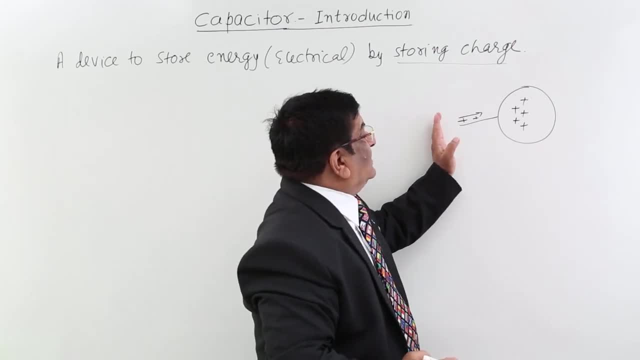 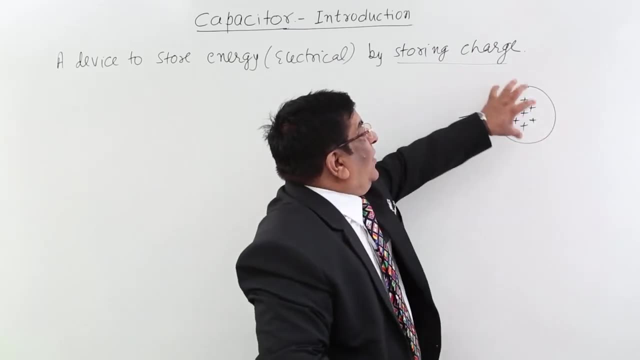 and I have to increase my force Again, increasing the force doing the displacement. I put them here. When I put and lock them here, then I have more charges. Then what has happened to my energy which I have spent in doing the work? 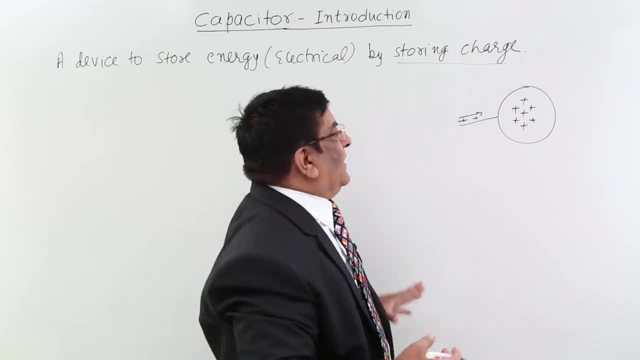 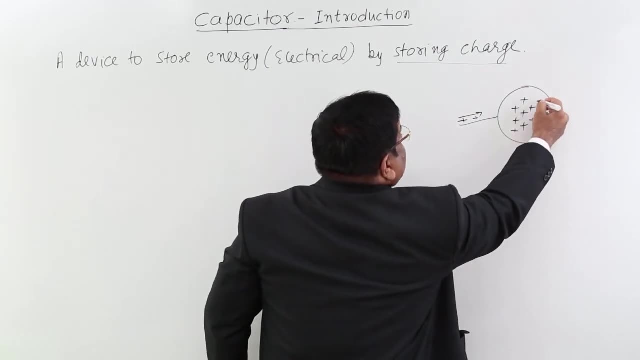 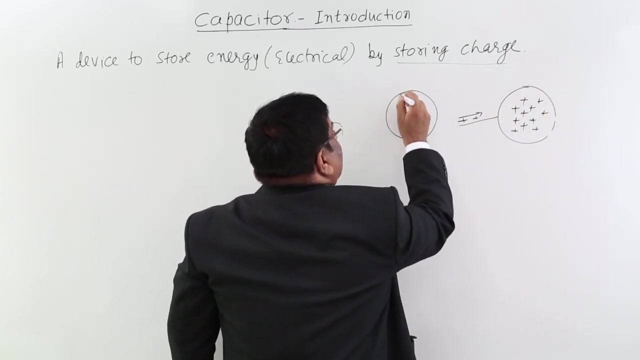 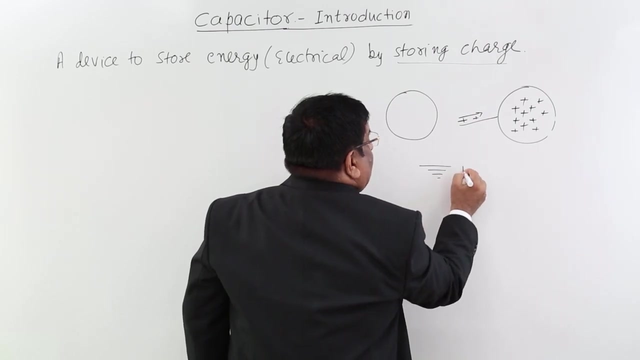 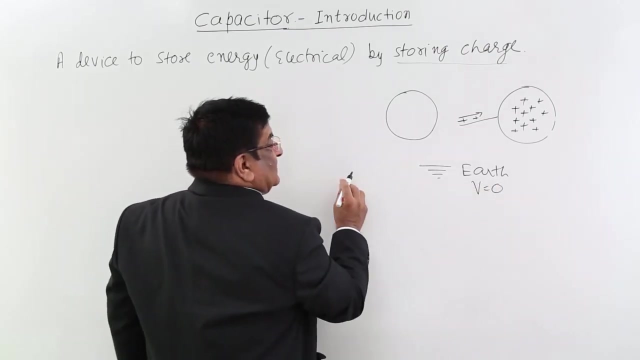 Answer that energy is transferred into this. Now another thing happens When we place charges here on this metal. a lot of charge is there Initially, when there was no charge, its potential difference with reference to earth. For earth we take as potential zero For infinity potential zero, For earth potential zero. So with reference, 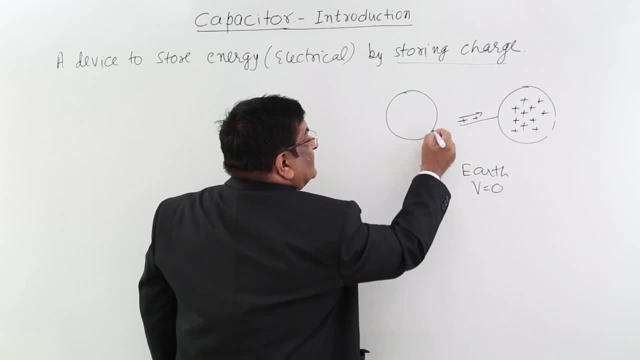 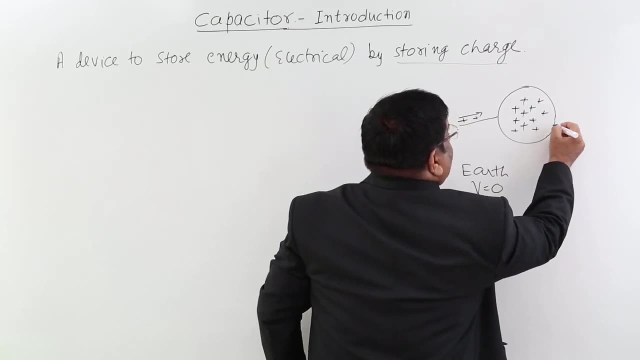 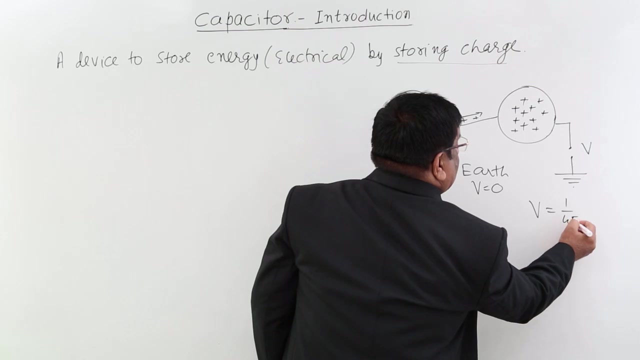 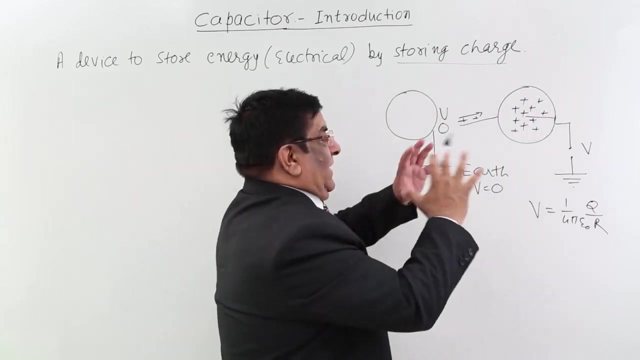 to earth. its potential difference was zero. Now, when I see the potential difference between this body and earth now, I find it has gained a lot of potential. How much is that potential, That potential? we know the formula 1 upon 4, pi, epsilon, naught, cube upon r. This is the potential of a ball, of a sphere, of any material. 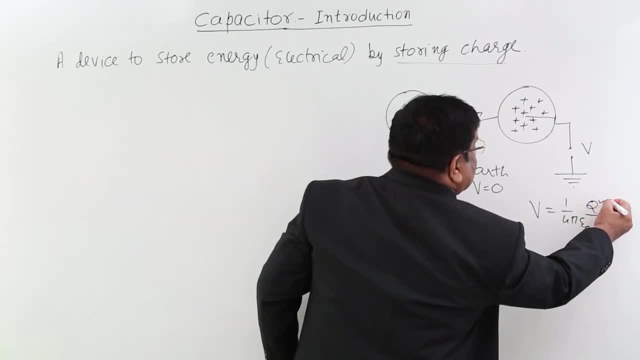 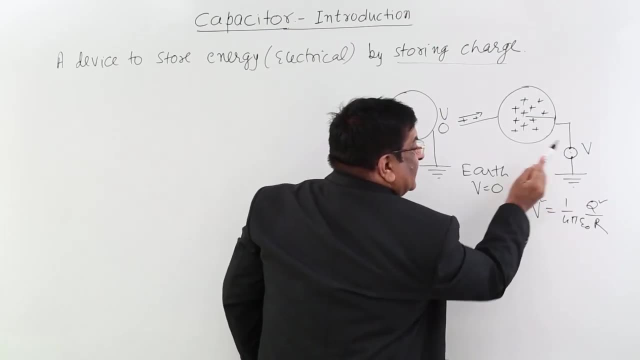 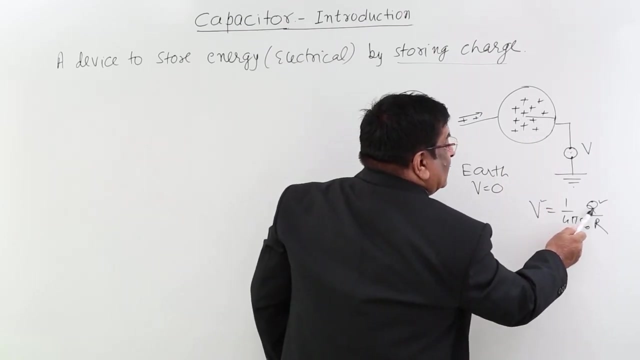 This is the potential. Now, if this charge is increasing, what will increase Potential? If I put a potentiometer here, if I put a voltmeter here, this will show a potentiometer here And this will show show me that this voltage goes on increasing. Why the voltage goes on increasing? Because 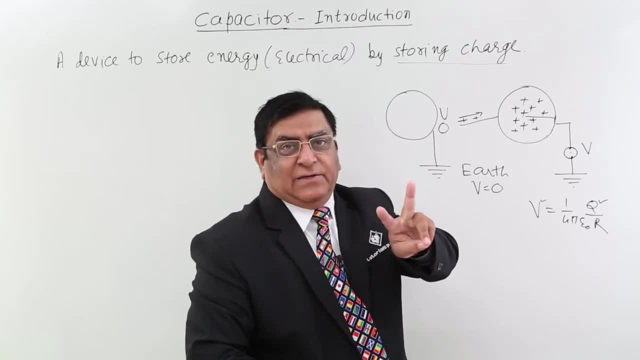 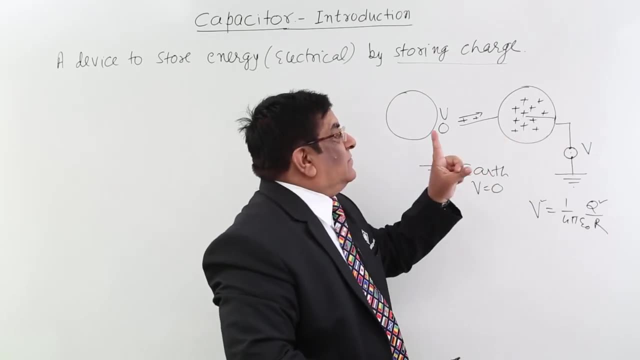 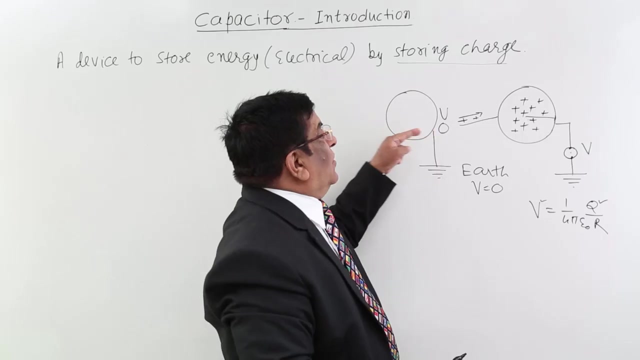 I am increasing the charge. I cannot see with my eyes the charge is increasing, but I can always see the voltmeter. If the voltmeter indicator is increasing, what is this indication for? The charge is increasing. So I am giving charge to it and I see the potential is increasing. 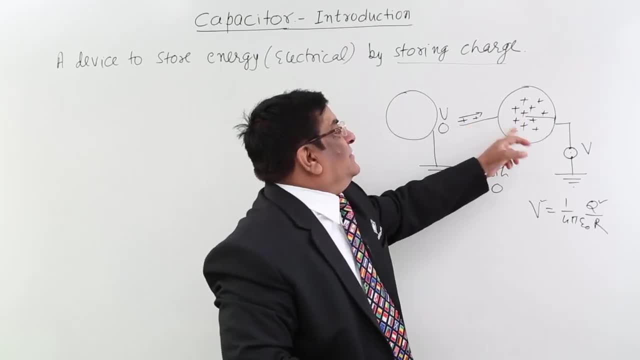 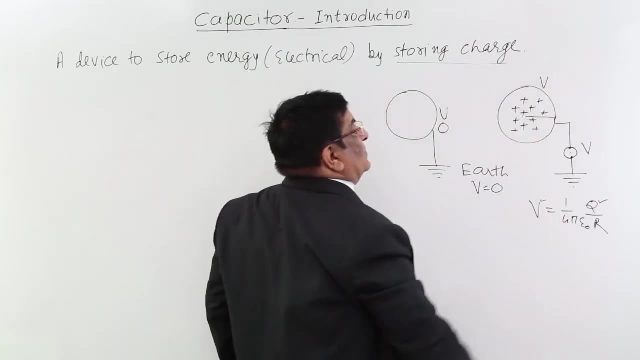 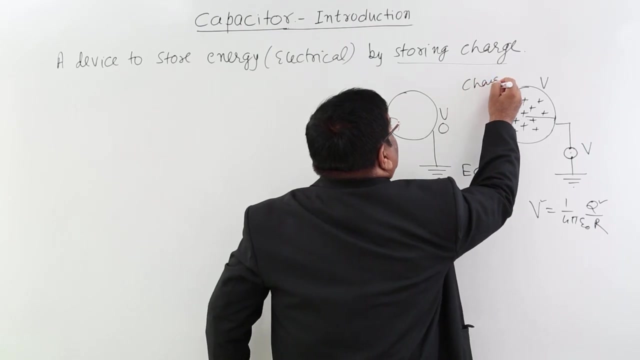 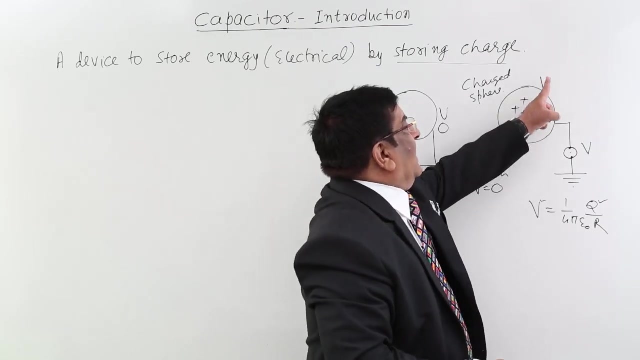 and now I can understand that my energy is being stored here, after sometimes I stop, and this potential has increased to V, and now I say this sphere is a charged sphere. This charged sphere is carrying charge, is at a higher potential and it contains all the energy. 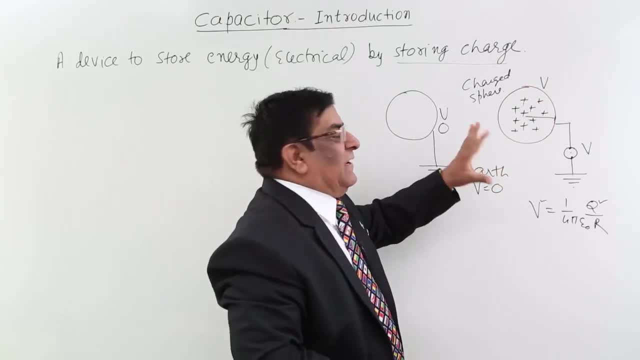 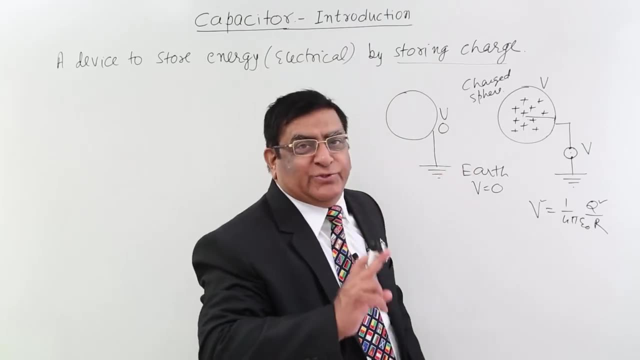 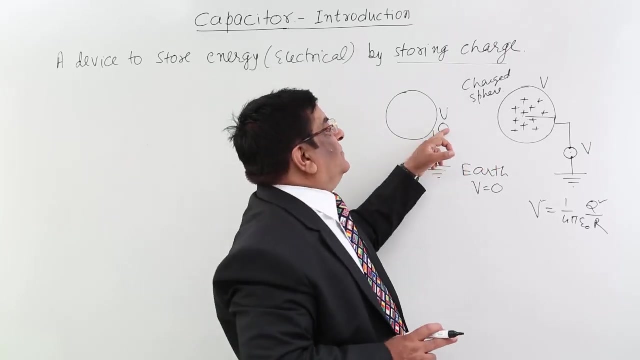 which I have given to it. Suppose we will calculate it, how much is the energy stored in it later. but now you can understand that V are in a position to store energy to a metallic plate if we have a device by which we can transport charge here by pressing it Like I can connect it. 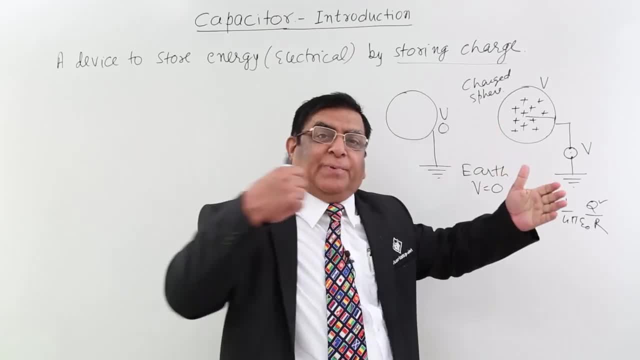 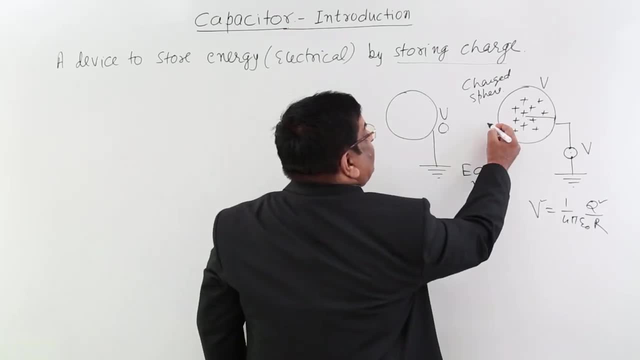 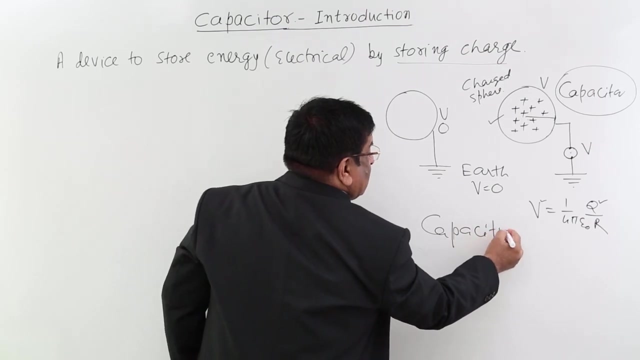 with a battery. I can connect it with a dynamo which will press charge into it and their energy is transferred into this material energy. and, friends, this is capacitor. why? because it has a capacity to do the work, capacity to do work, who can do work, who has energy. 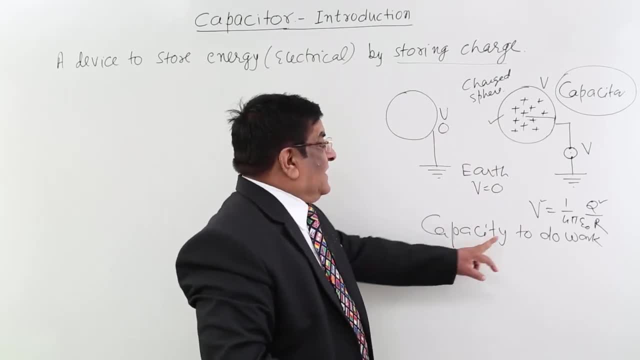 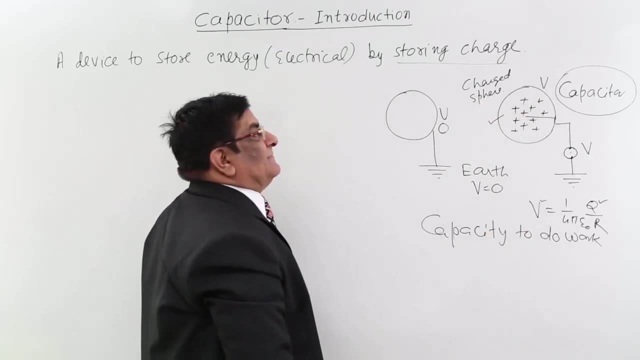 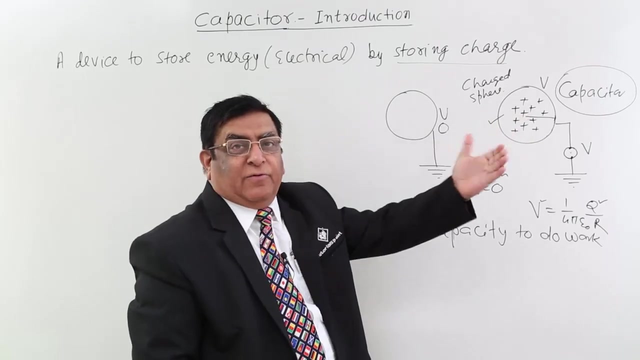 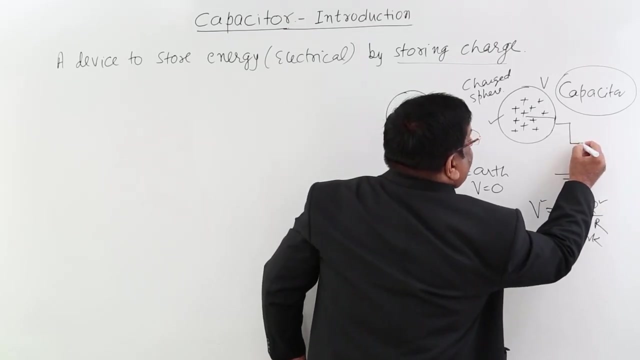 so this has energy. ok, so this has capacity to do the work and therefore this is a capacitor. so this way, now, if i want it to work to give back my energy, what i will do here, i will put a bulb and connect it with the earth, which is V is equal to 0, its potential is V is equal to V. This is high potential. this. 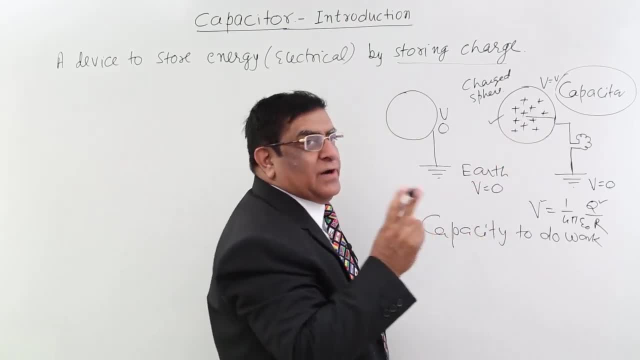 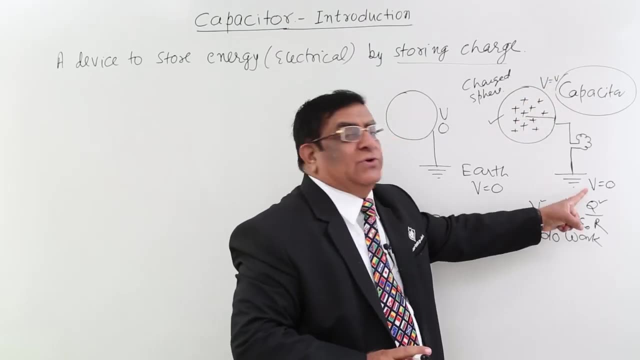 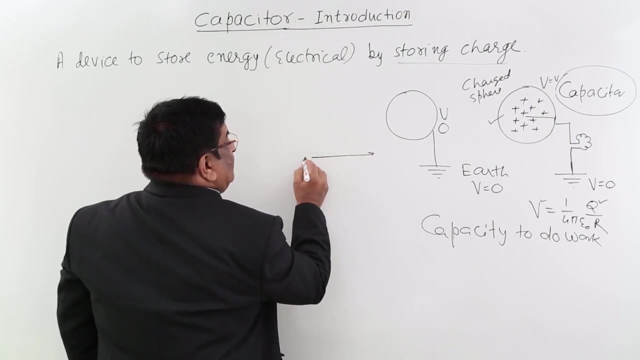 is low potential and we have learnt, or remember it now: a charge. they will repent each other and they will flow from higher potential to lower potential. I will remind you once again: if this is electric field here, what does it mean? There is a body here with positive 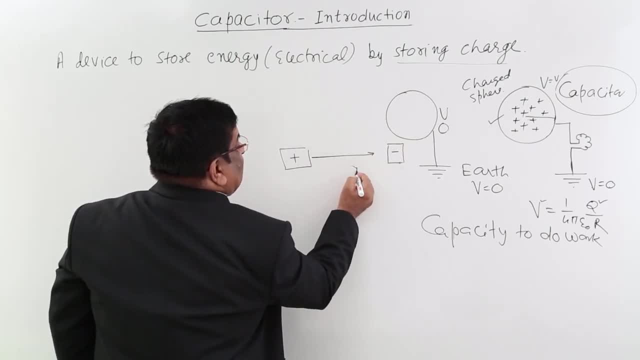 charge a body here in negative charge. So this is direction of electric field. If this is direction of electric field, then there are these equipotentials, V, V lines or equipotentials. This is higher potential, close to it, lower potential, lower potential, still lower potential. 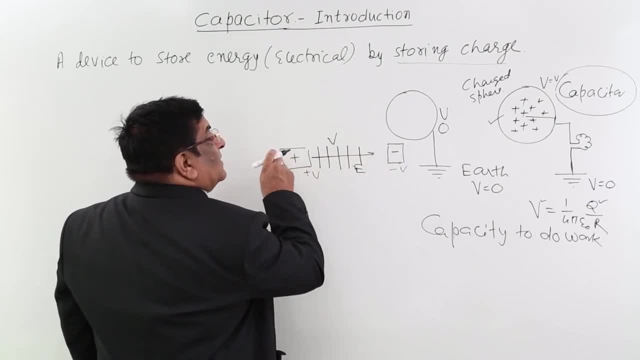 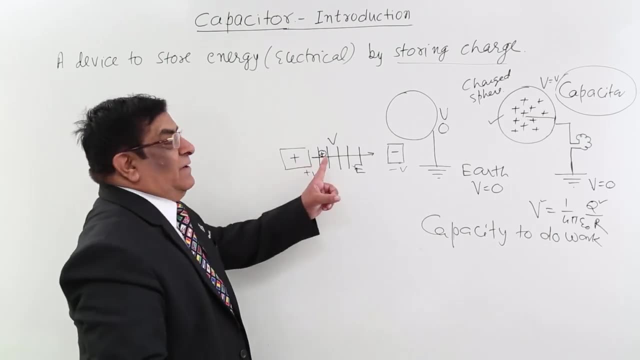 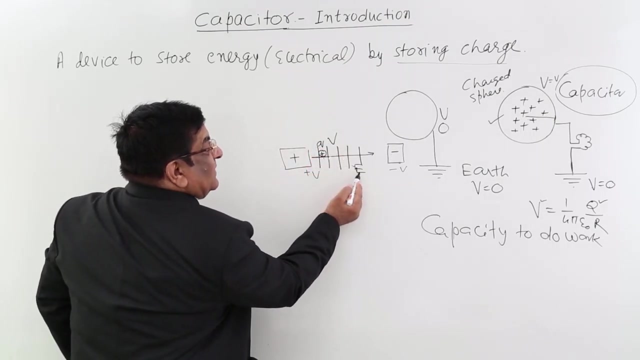 negative potential. So this is: the potential is decreasing in this direction. Now I place a positive charge here. What will happen? We can learn it by two methods. Number one: this charge Q will experience a force because of electric field and this force is: 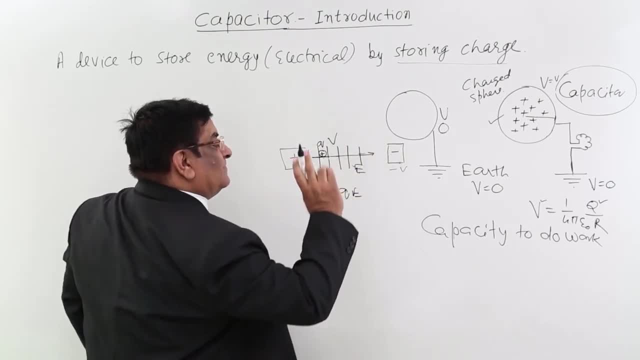 QE. Because of this force, it will move like this Other. due to repulsion, it moves like this. So I say: a charge moves from higher potential towards lower potential. This is, you must remember it, It is a thumb rule, With charge positive Whenever we. 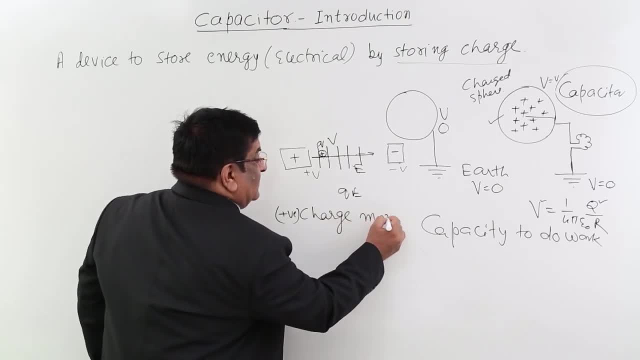 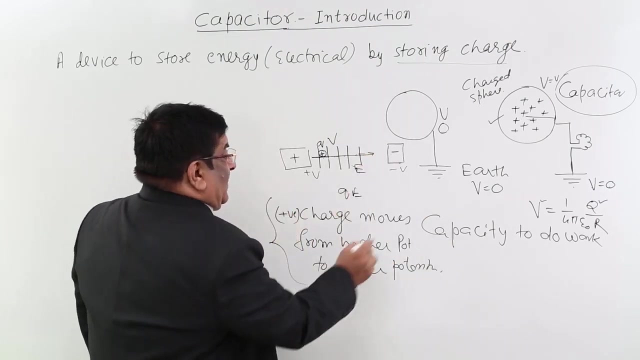 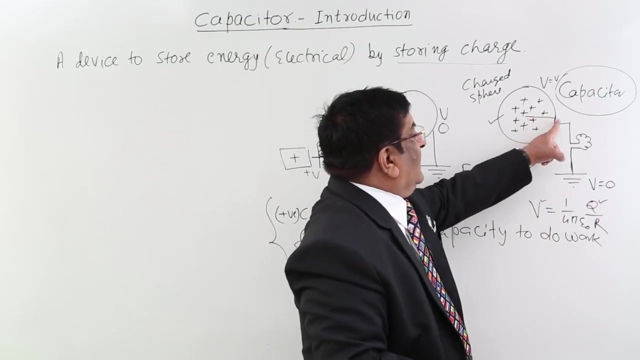 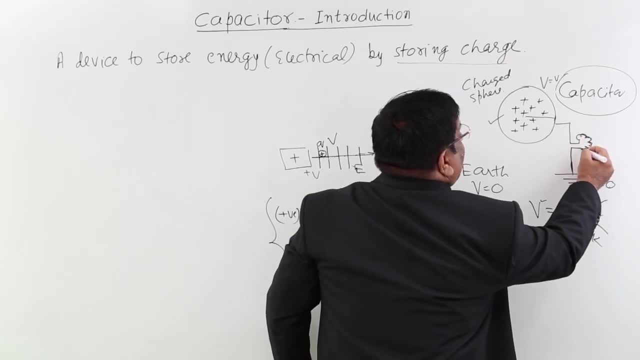 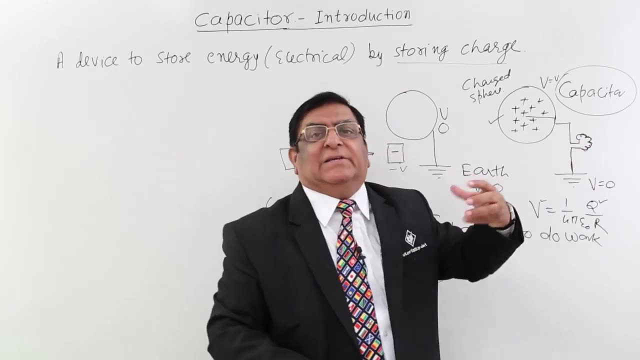 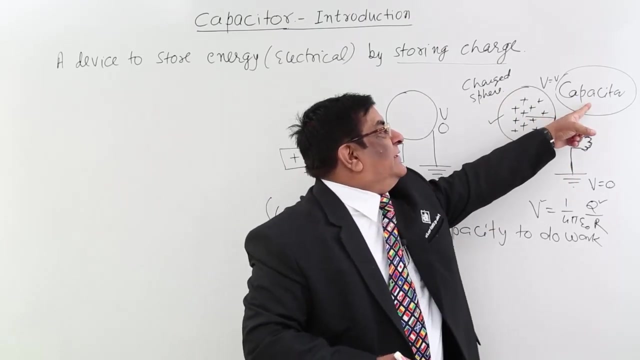 the charge moves here, it has to go through the bulb and the bulb brighten up. We get the light from the bulb. Getting light from the bulb is bulb is working because somebody has given it energy, Who has given it energy? This and what we call it Capacitor, because 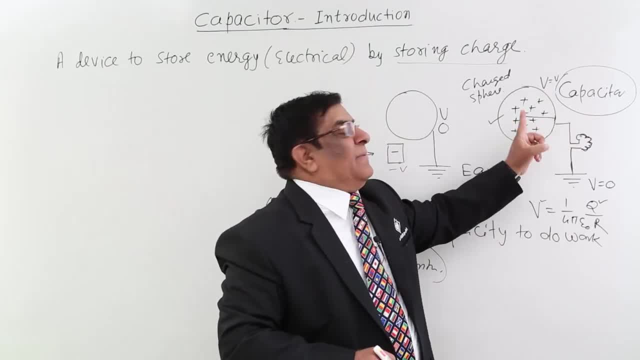 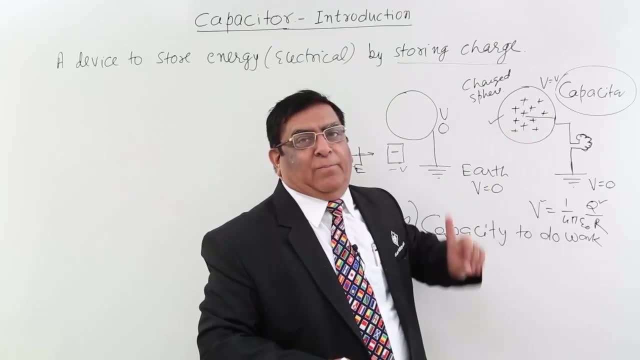 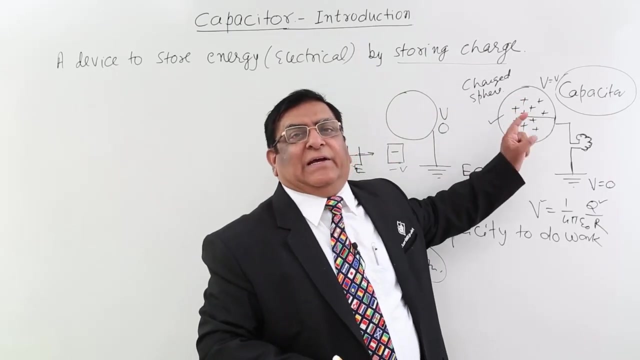 it has capacity to do the work. So what does a capacitor do? Capacitor is capable of creating resistor, stores energy. and what is this made of? this is made of metal plate. how does it store energy? we press charge into it and whatever work we do, that energy is stored in it. what